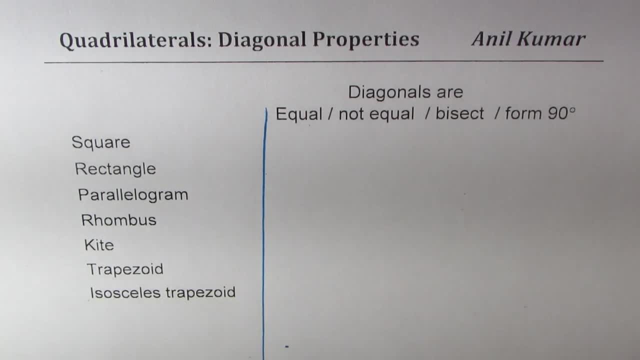 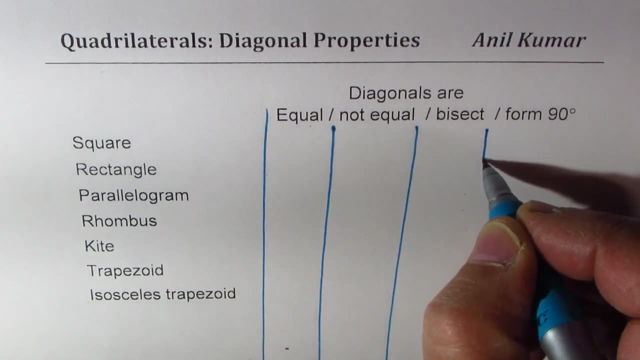 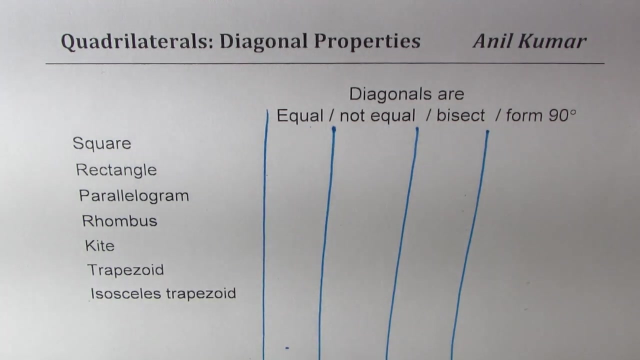 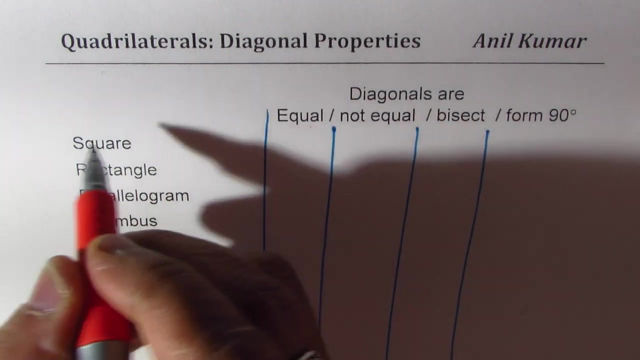 criteria that if we have diagonals, whether they are equal or they're not equal, do they bisect or they don't bisect? And at what angle do they bisect? Is it 90 degrees or not, To begin with, if we take a square, for example? so if we take a square, let me draw here: one square means all sides are equal, right? So we 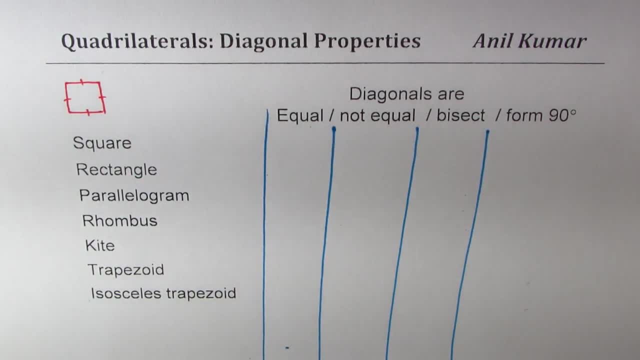 mean all sides are equal. So in this particular case, if I draw the diagonals, then both diagonals are of same length, they bisect each other and they are also at 90 degrees, correct? So they are at 90 degrees, correct. So in this particular say, we will say that in case of square, diagonals are equal. 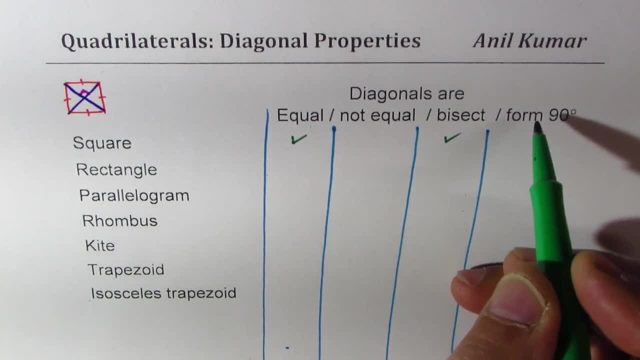 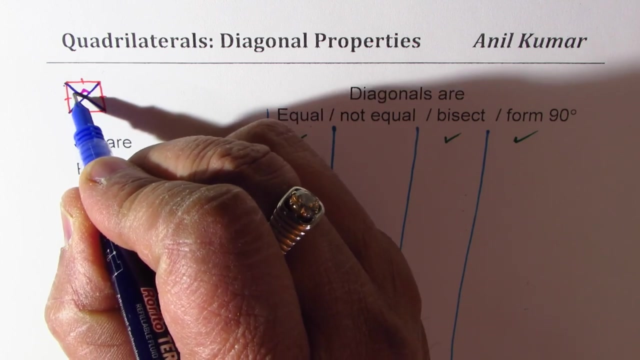 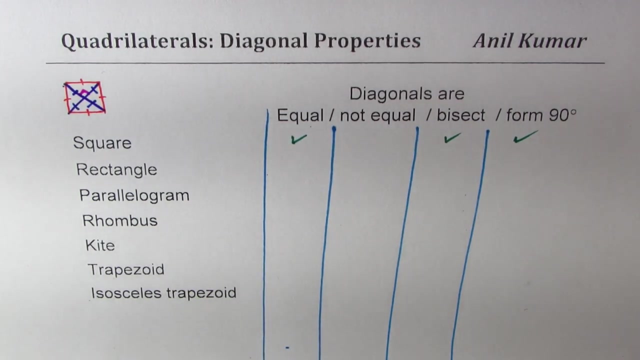 right, And they bisect each other and they form 90 degrees. That is what, in short, we are going to write. Does make sense to you? Perfect. So this really means that equal means these two lengths are absolutely same. we can say: all of them bisect, so they are all equal segments, Perfect. Now if you take a rectangle? in that case, what happens? 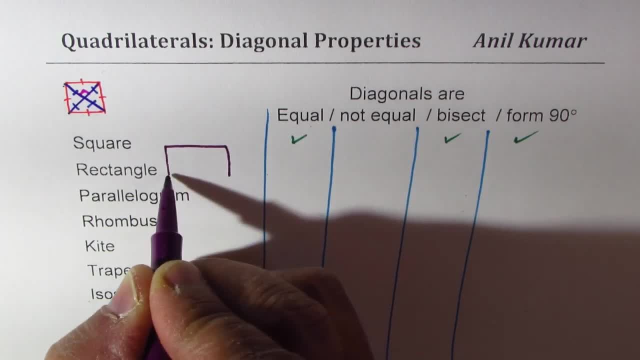 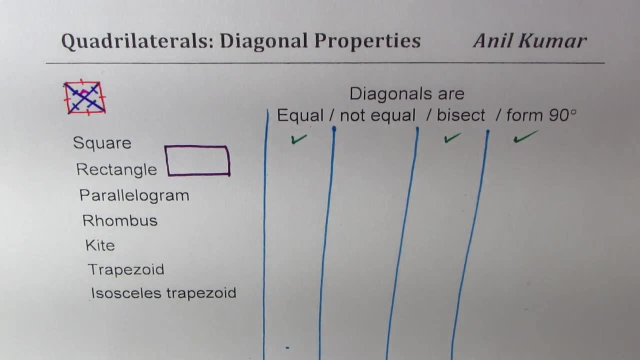 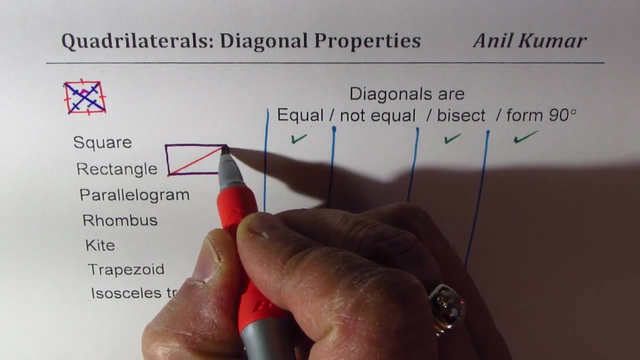 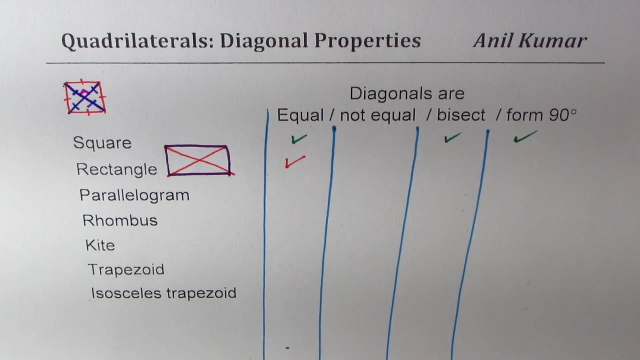 What I would like you to do is pause the video at this stage. copy this table, do it yourself, right, And then compare with my results. That is going to help you to understand the concept. Now, in this case, we see these two diagonals. so they are equal, correct, Their length is same, So we say they are equal. diagonals are equal in a rectangle. Do they bisect each other? That is, do they bisect each other? 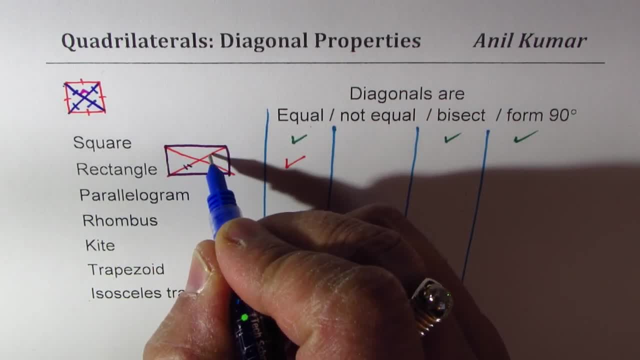 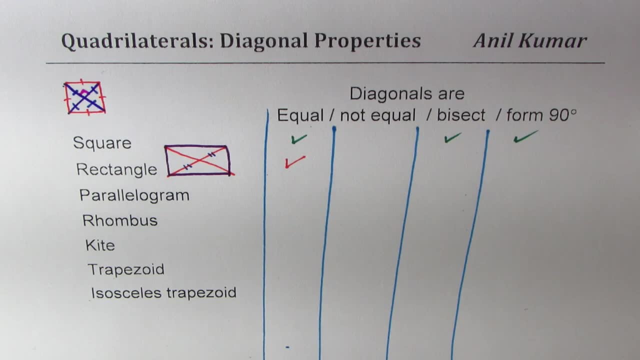 to say that this point is an intersection and so all these lengths are indeed equal. So when you have a rectangle, in that case, as in the case of square, they do bisect each other. So, yes, they do bisect, but do they form 90 degrees? No, they don't, As you can. 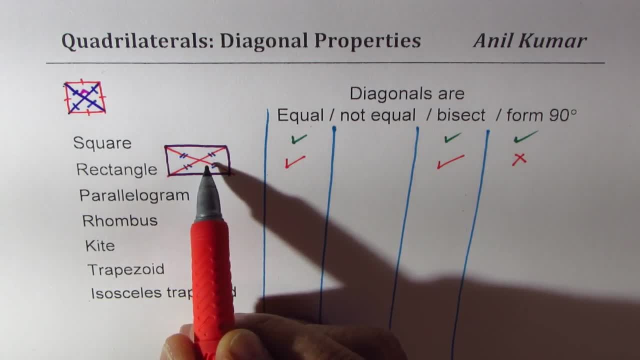 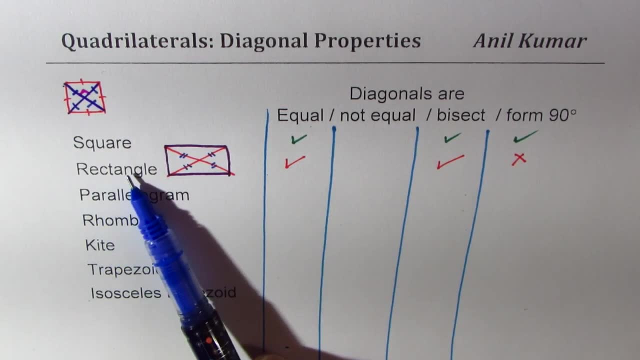 clearly see the angle is: one of them is greater than 90, the other one is smaller. So when we talk about rectangles we'll not consider squares. Squares we have taken separately, So don't mix up into those issues. So we know all rectangles are parallelogram, but when 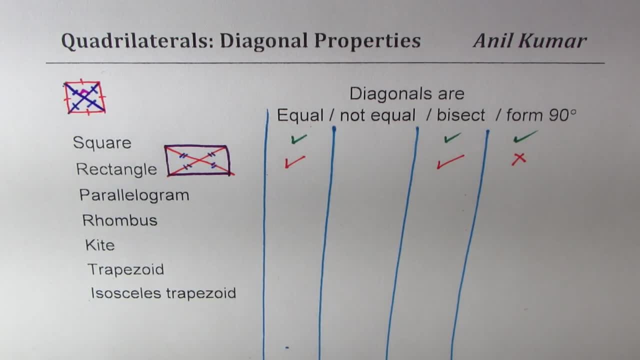 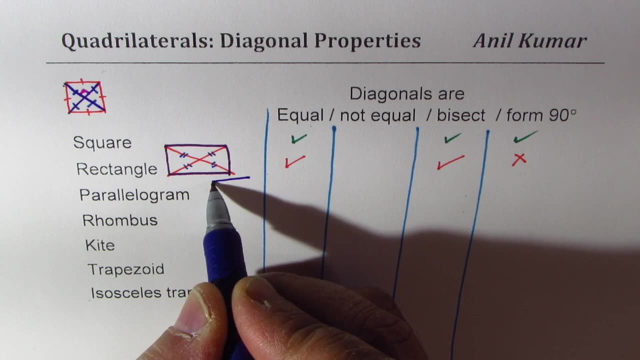 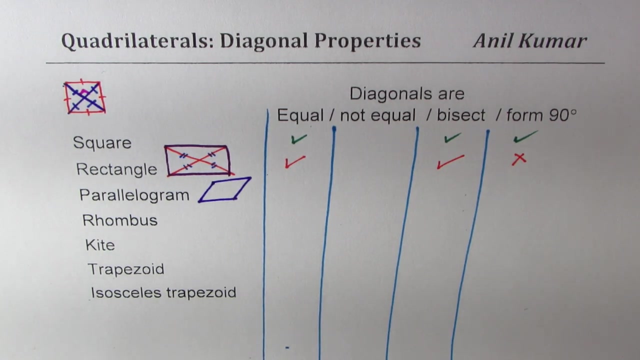 we say parallelogram, that means not a rectangle, Is it clear to you? Now let's talk about parallelograms. So where the two pairs of parallel sides are there, kind of like this: right lengths are different. Now, in this case, what do you expect about the diagonals? So let's say: 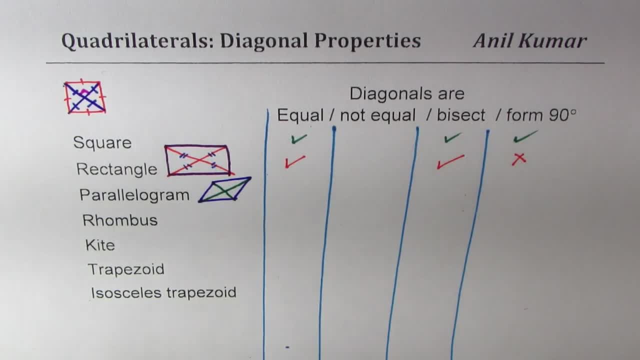 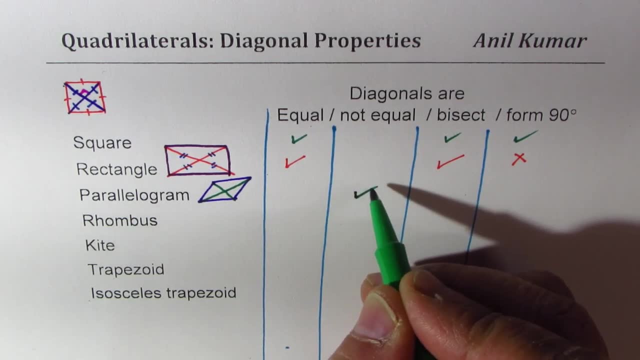 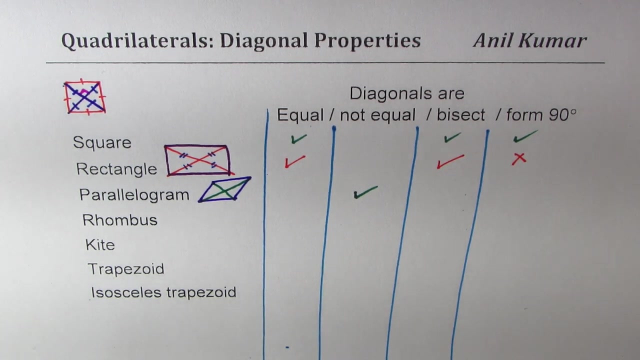 these are the diagonals, So one is longer than the other, right. So clearly, in case of a parallelogram they are not equal right. So I'll put not equal. the diagonals are not equal. Now do they bisect? 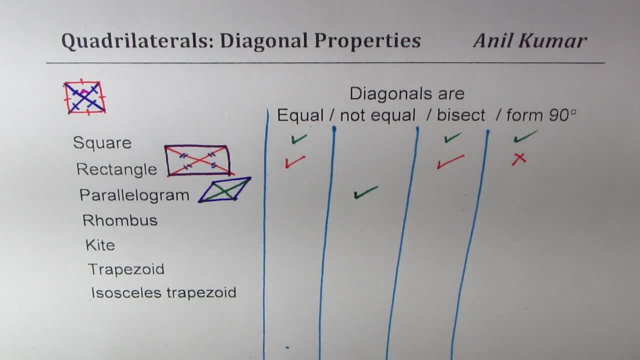 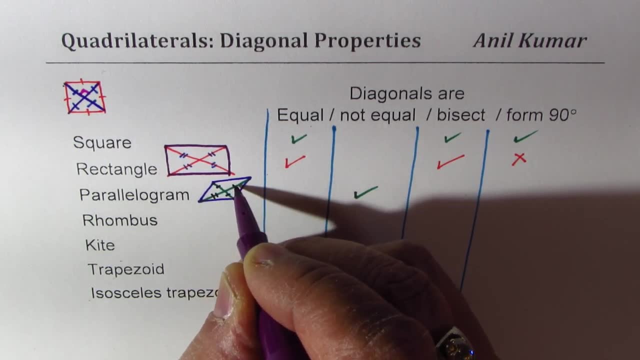 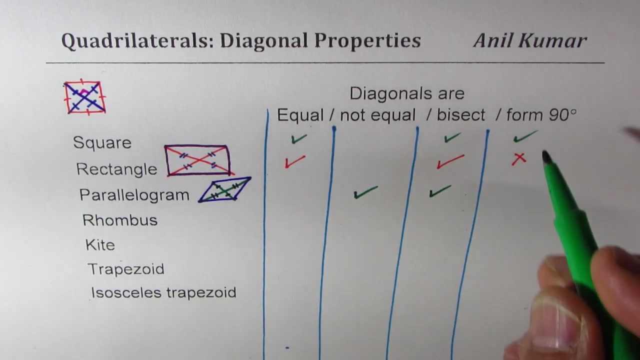 So you will see that in parallelogram. they are not equal, but they do bisect each other. So we have this side equal to that and this portion of the diagonal is also equal. So they do bisect. however, again, they do not form 90 degrees. 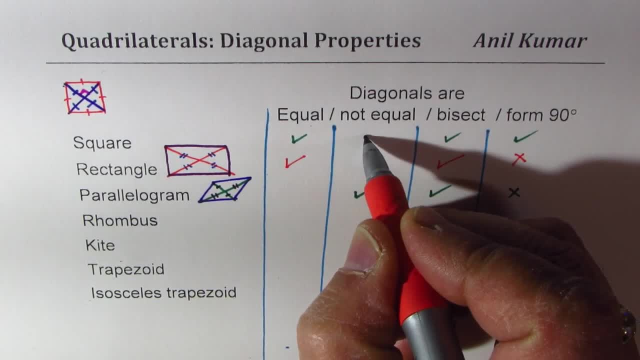 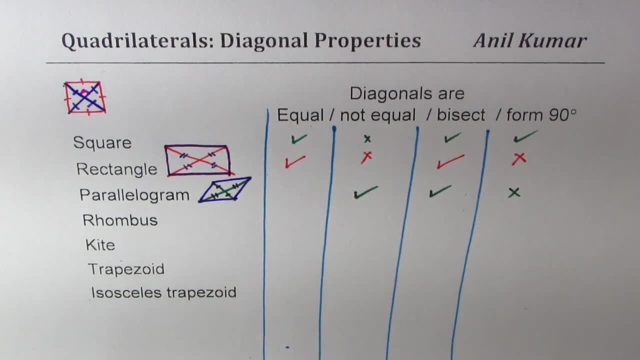 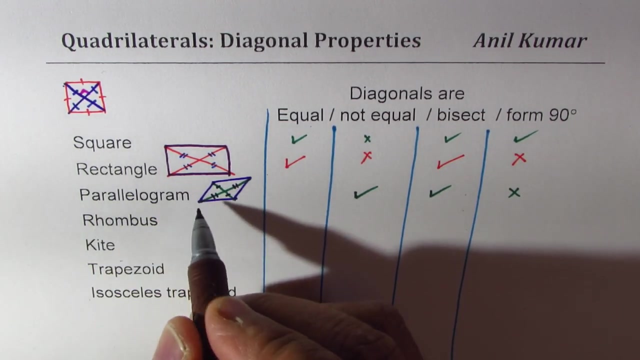 So I am writing not. So let me just say here also: not equal to and they are equal. so therefore not equal will be cancelled. Now, if you consider a rhombus, rhombus means kind of a parallelogram with all four equal. 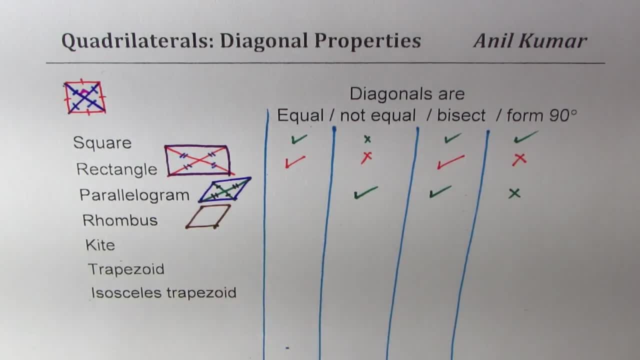 sides. So all four are equal in length also. So in rhombus, what do you expect? Are the diagonals equal or not? Do they bisect each other or not? So rhombus is not a square, but it does have all four equal sides. 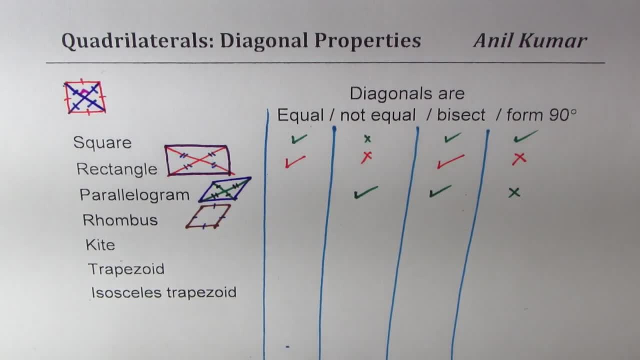 Now, what do you think? Do they bisect at 90 degrees? This is what you need to answer for rhombus, Let's check. So if I have these two diagonals right there, Clearly you can see that they are not equal. 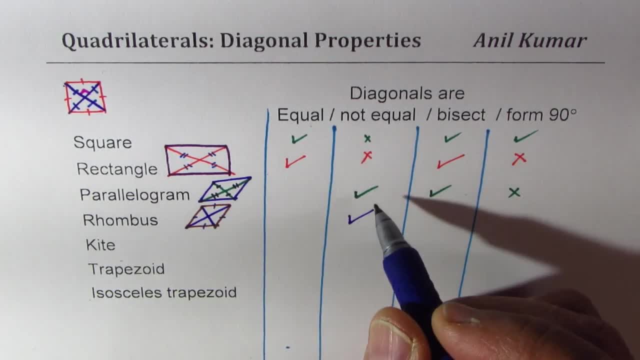 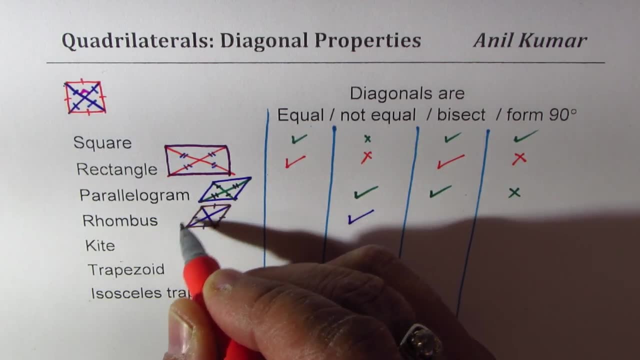 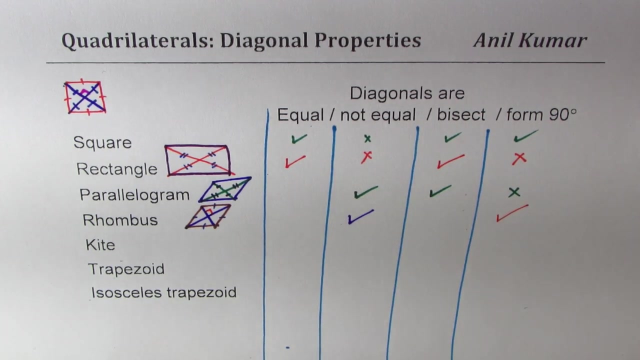 So they are not equal. One of them is longer than the other, But since all these sides are equal, you will notice that they actually bisect each other. So, as far as the intersection is concerned, they do bisect each other at 90 degrees. 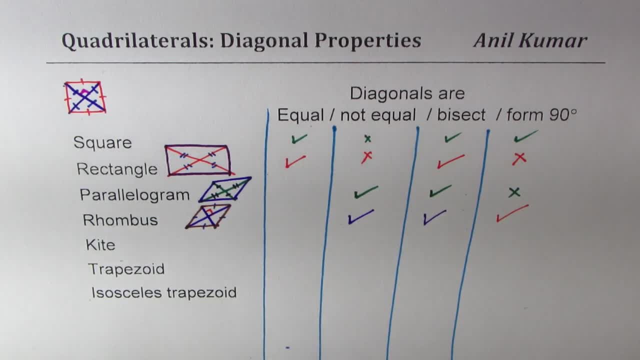 So they do bisect. also, they are at 90 degrees. So that is unique about the rhombus, But the diagonals are of different length, Correct. Now let's consider the kite. When I say kite, it means we have a structure which is kind of like this: 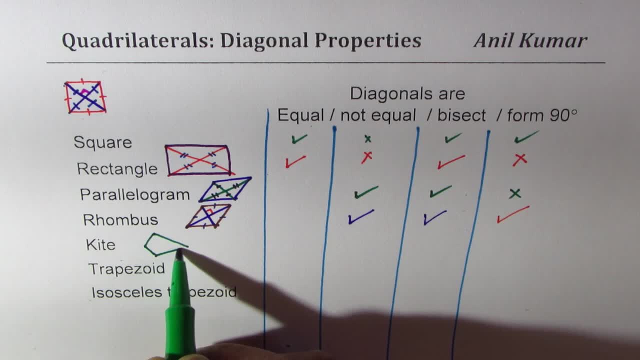 Two sides of equal length, right, Kind of like this. Do you see that portion? So this is a kite In a kite. these are my diagonals. These diagonals always intersect at right angles, Correct? So as far as right angles is concerned, yes, they do intersect at right angles. 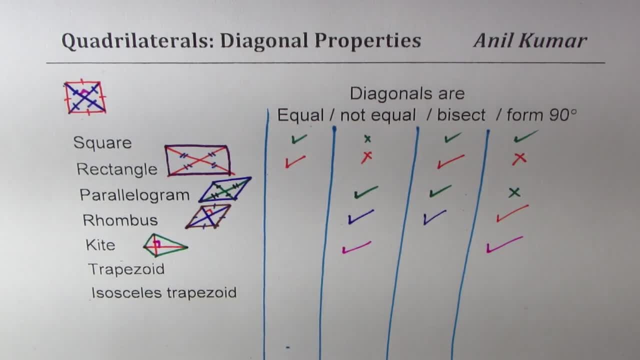 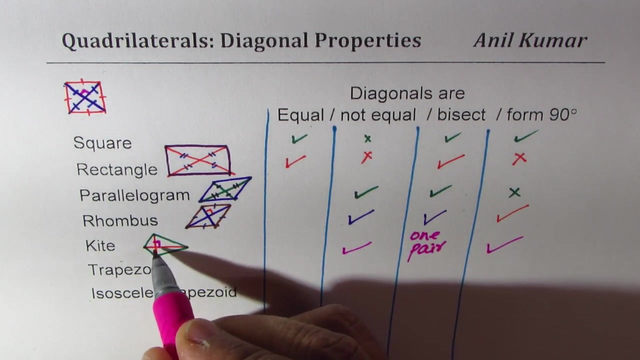 And clearly they are not equal. One is smaller than the other. And how do they bisect? Now, what do you notice here is that one pair is bisected, So only one pair. So you see that smaller one, in this case, is being bisected. 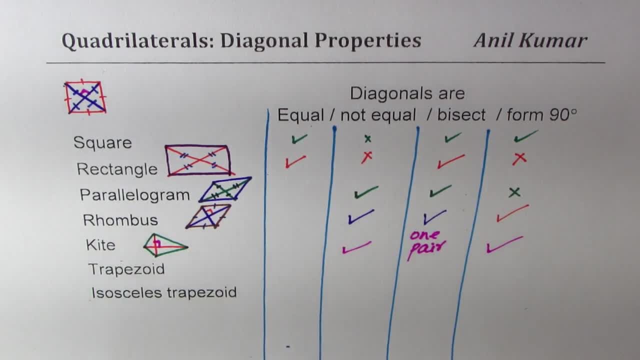 Not the other one. So one pair is bisected. So that is kind of important to see in case of a kite. Now, when we talk about trapezoids, I could have a trapezoid which is called isosceles trapezoid. 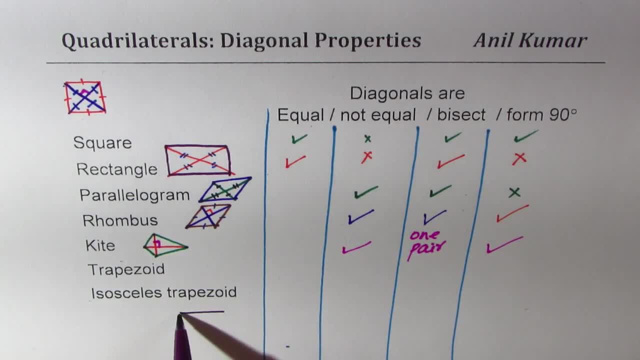 So in isosceles trapezoid- let me sketch one here We have- these two sides are parallel, However these two are equal in length. So in case of an isosceles trapezoid, what you notice is that the diagonals, they bisect. 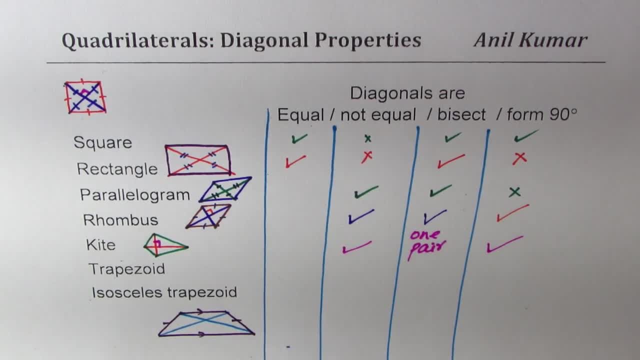 So these are your diagonals, correct? So what do you see? So they bisect, and in a different way, kind of How You will notice that this side is equal to that side and these two sides are equal, So in a very different way. 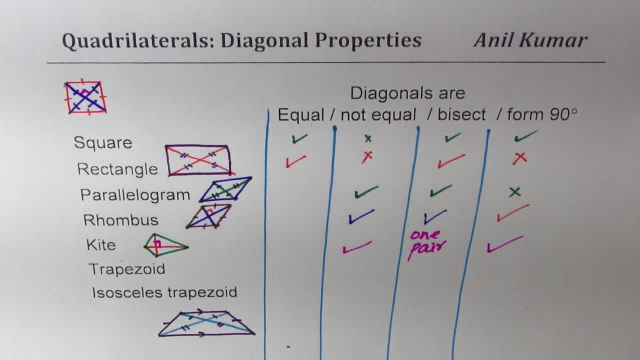 So they do have equal pairs of those lines. So in an isosceles trapezoid they are of equal length. So in this case they are of equal length In a normal trapezoid, which is not an isosceles trapezoid. 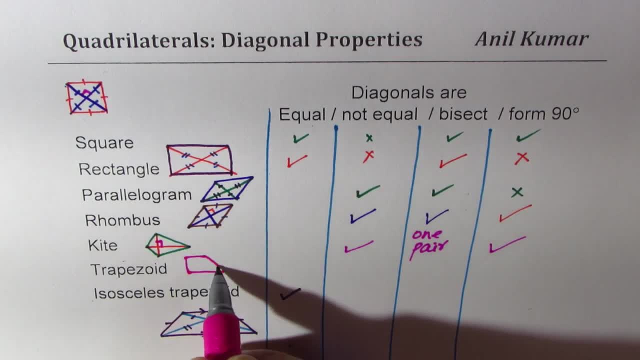 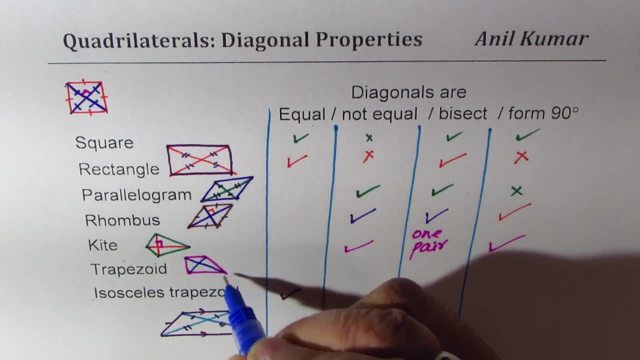 So let me just make one here, kind of let's say like this: So I am making one so that it is apparent That in this case diagonals are not equal. Right So diagonals are not equal. It doesn't make clear to you, right? 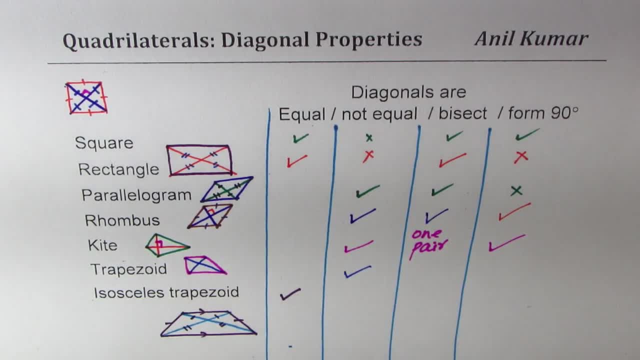 So diagonals are not equal, Is that okay? So if you make a normal trapezoid, not an isosceles trapezoid, In that case nothing is true here. I mean, these diagonals are not equal and they don't bisect each other, right? 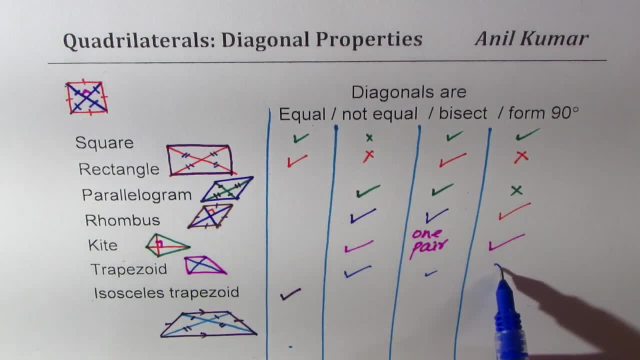 So in this case they don't bisect and they do not form 90 degrees also. But in case of an isosceles trapezoid, Both diagonals are equal Right. So they are not equal, Okay, And they don't really bisect, but they do have a pair of opposite sides. 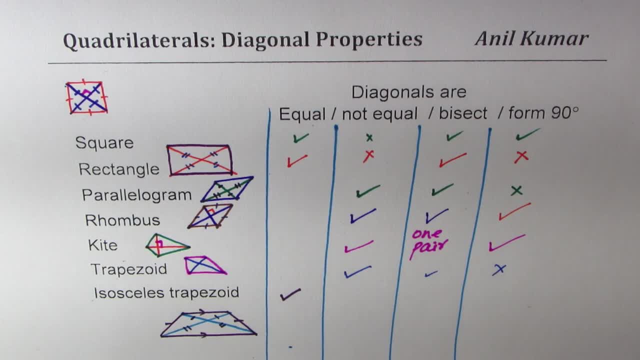 So what I am trying to say here is that two pairs of equal segments are there, These two right. So we have a special case here. So we have two pairs of equal segments Which are not equal Right, Which are not of one diagonal. 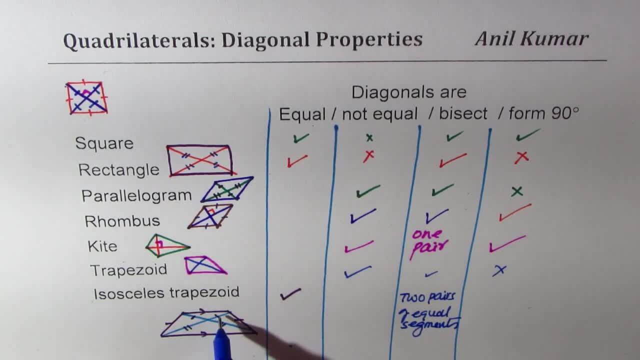 You know of both the diagonals- top, top, bottom, bottom. So that is what we are trying to say here. So I hope that makes sense. So I would like you to go through this list once again. Try to see which of these diagonals bisect, and that too at right angle. 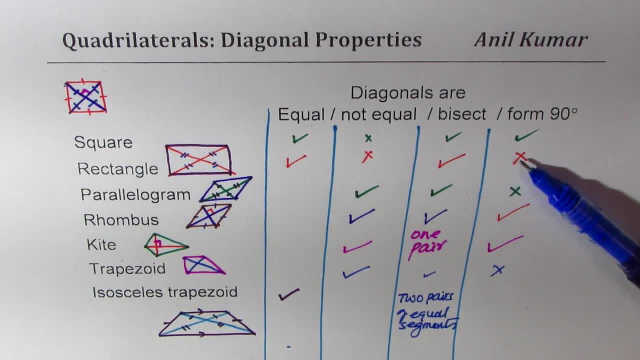 So, as we can see, those which bisect at right angle are square Right And rhombus Correct. So likewise, you can see a lot of similarities between quadrilaterals and the properties of their diagonals. Now for you, we have a test based on this learning. 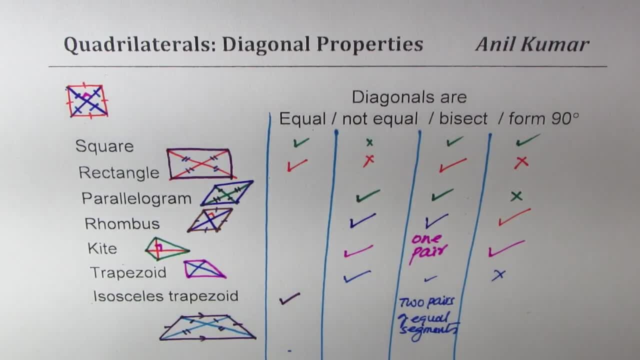 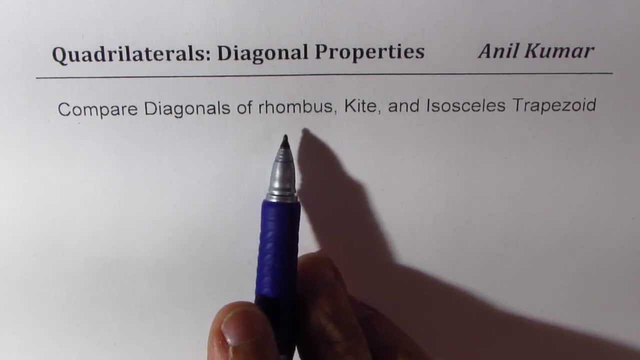 So let's move on and take the test on diagonal properties of quadrilaterals. Now here is a test question for you. You need to compare diagonals of rhombus, kite and isosceles trapezoid So you can actually pause the video. 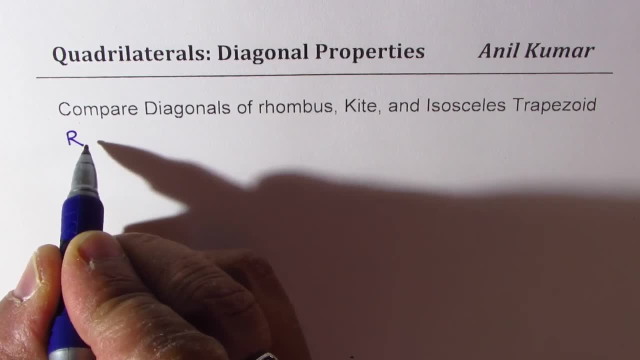 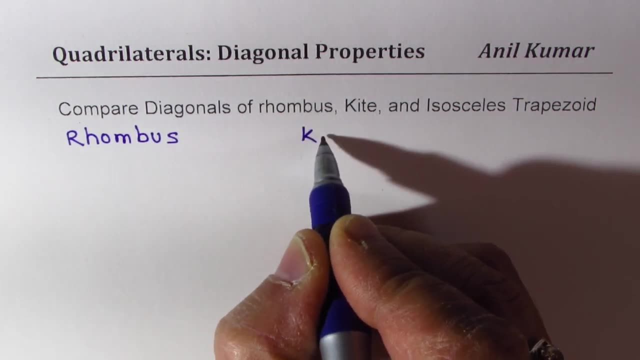 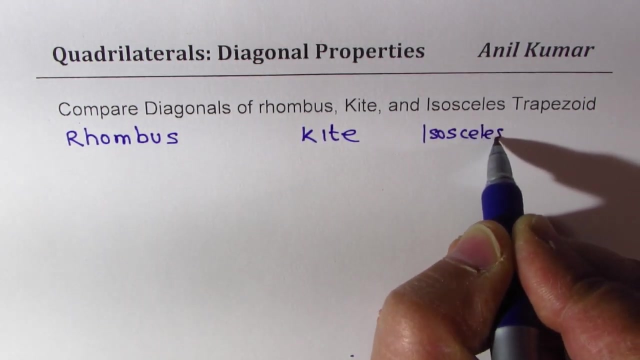 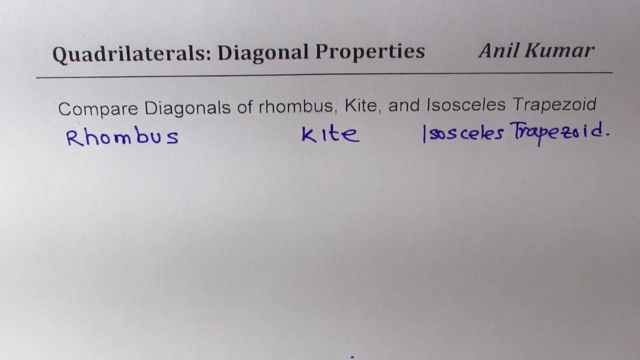 Okay, Pause the video, write the answer and then check with my solution. So we'll sketch rhombus. we'll sketch a kite and isosceles trapezoid And then we'll compare them. So rhombus really means that it's kind of a parallelogram. 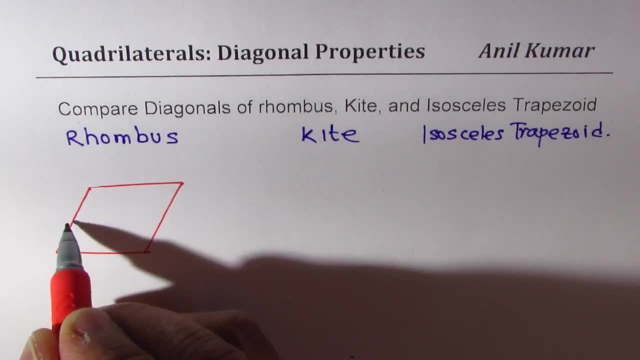 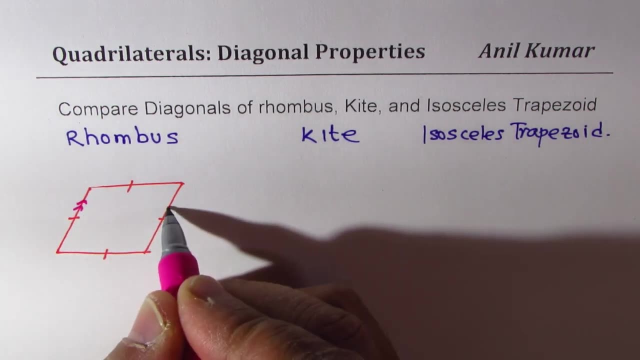 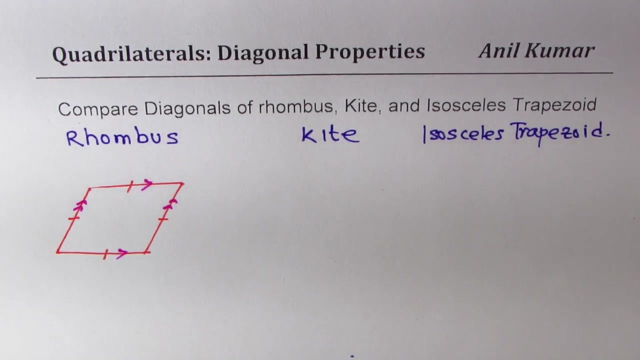 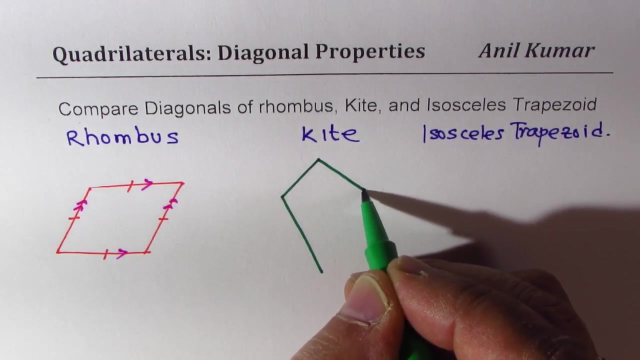 With all four equal sides. So when I draw like this, we know these sides are all equal and also they are parallel. That is a rhombus. As far as the kite is concerned, it will have one pair of equal sides on each end, and isosceles. 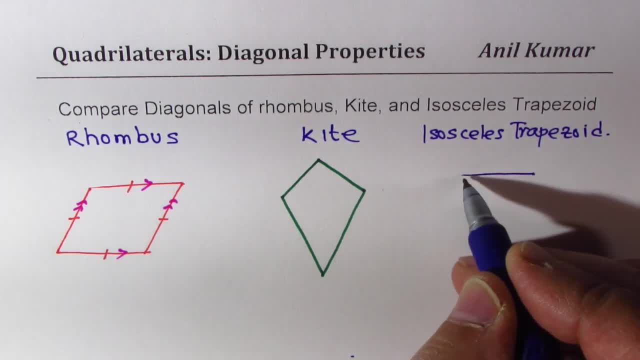 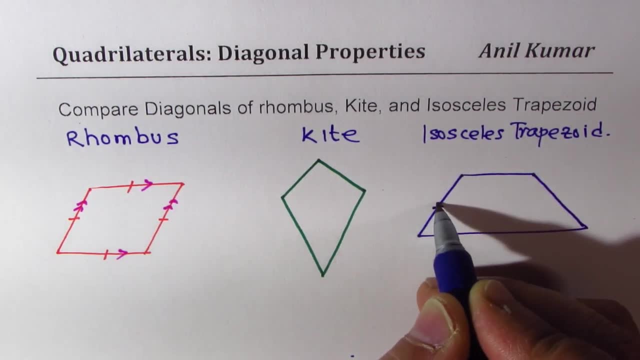 trapezoid, We're trying to make bases parallel and the sides equal, So that is an isosceles trapezoid. So what I would like you to do is to write the properties of diagonals in these three two dimensional shapes. 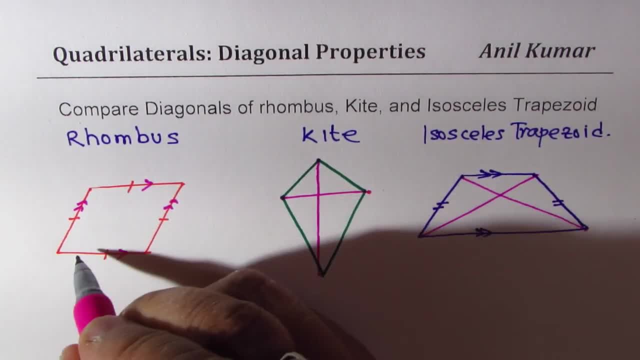 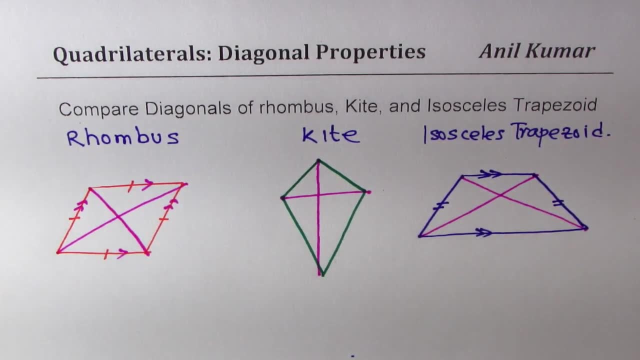 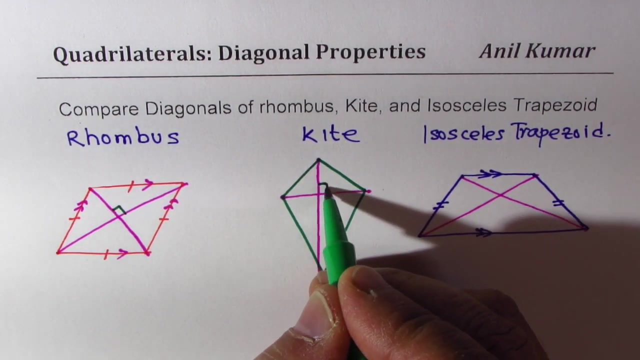 So do they bisect each other? Yes, Yes, Do they intersect at 90 degrees? That is what you need to answer, Correct? So, as we saw, this intersects at 90 degrees. This also intersects at 90 degrees, Correct? 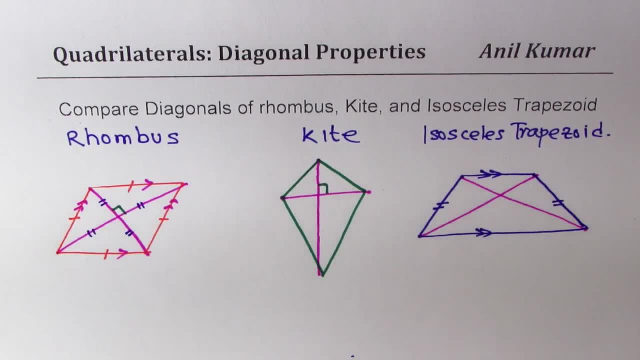 Here all four sides are equal. In this case one of them- pairs is equal, Correct. In this case, these two portions are equal, the other two. Let me write three lines here. Do you see that portion Correct? So that is how.